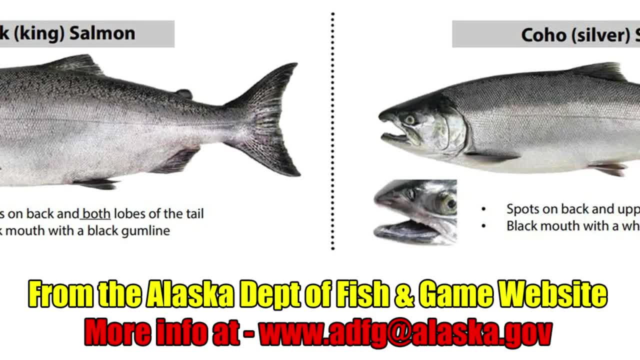 They have a thick, round, thorny gill fin and a large, pointed and pointed tail, which is often referred to as the silver-sour jaw. Smaller, younger king salmon are easily confused with silver salmon, which is why the unique 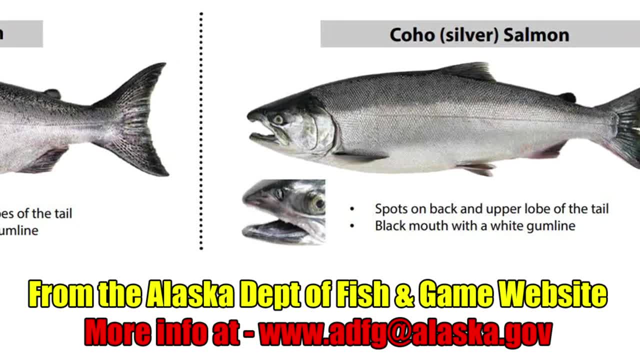 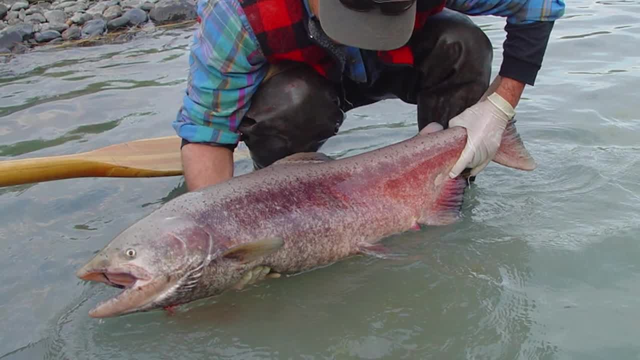 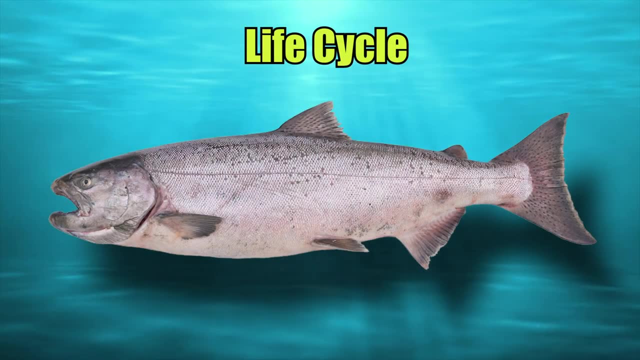 feature of the black mouth and black gum is so important for identification. When king salmon spawn, they darken in color quite dramatically and turn into a dark olive or maroon color. King salmon are born in freshwater rivers and hang around for about a year before heading. 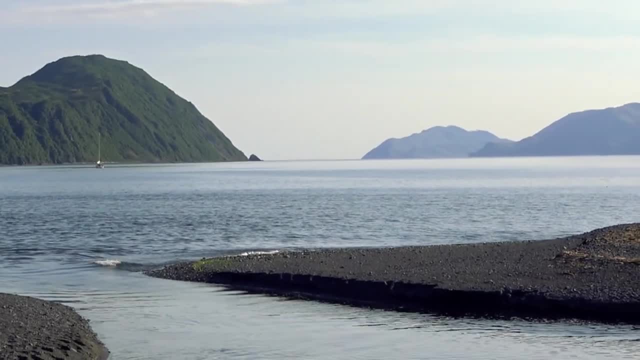 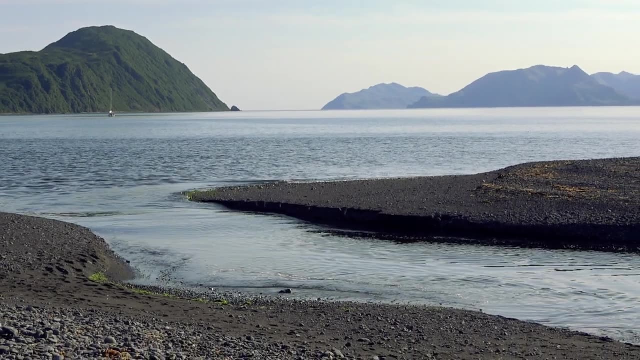 out to saltwater. From there they can be found in the wild, the mountains and the waterways. Kings then spend one to five years out in the ocean, feeding and growing, until heading back to the freshwater river of their birth to spawn and then die. 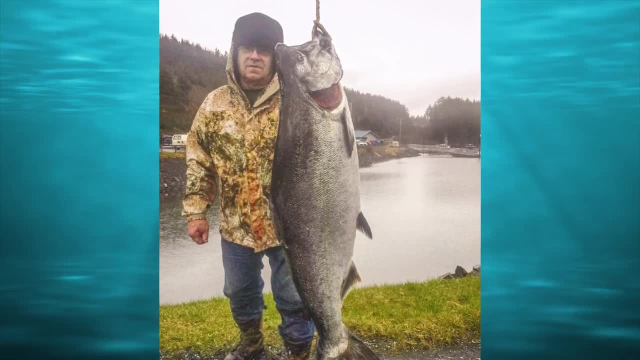 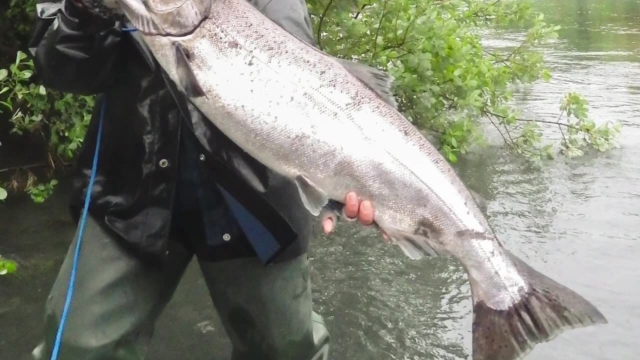 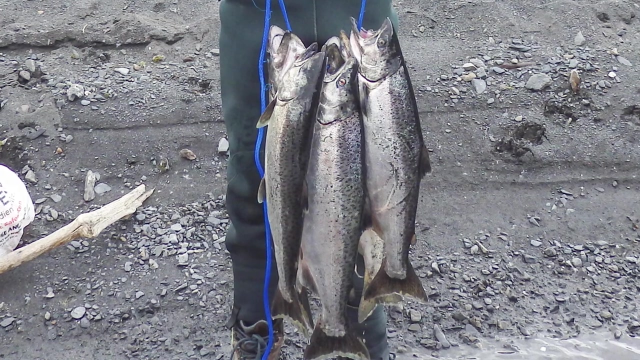 King salmon grow rapidly and can double their weight in just one summer. They eat a variety of different foods, depending on their stage of development, including plankton, insects, smaller fish, squid and crustaceans. Small king salmon that return after only one year out in the ocean are referred to as jacks. 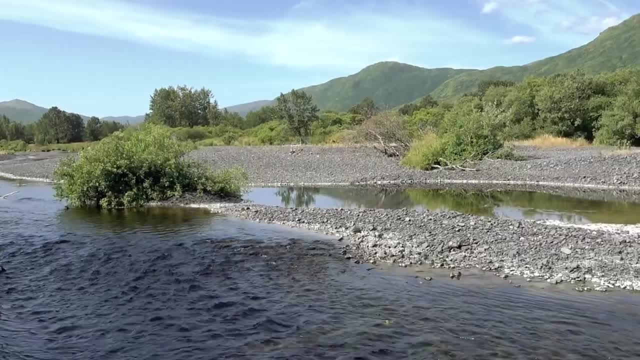 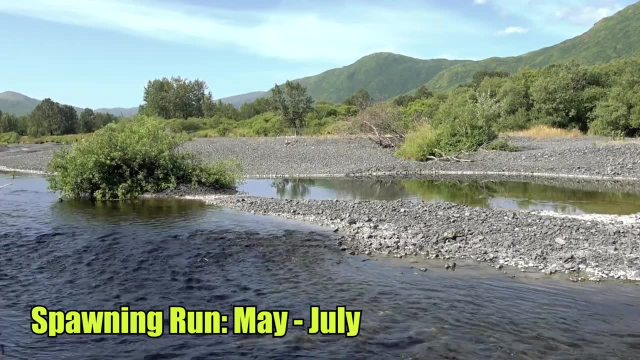 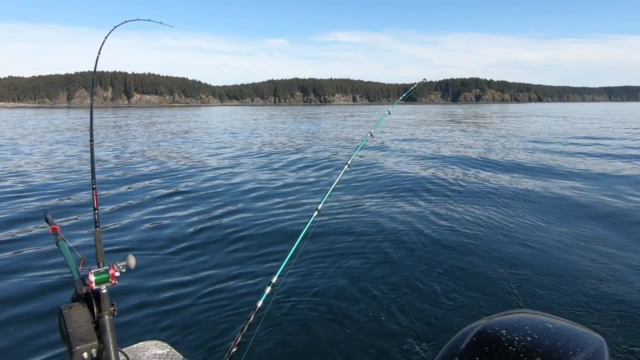 and they're usually male fish. Most rivers in Alaska that support king salmon usually just get one run of spawning fish, which happens sometime between May through July. King salmon can be caught with a variety of fishing methods and tackle: from trolling out in the deep waters of the ocean, fishing from beaches where kings move through, and. 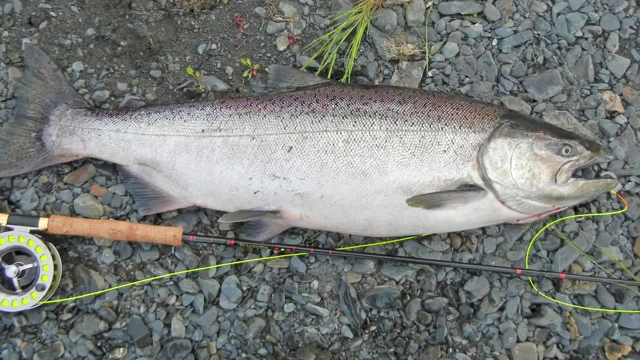 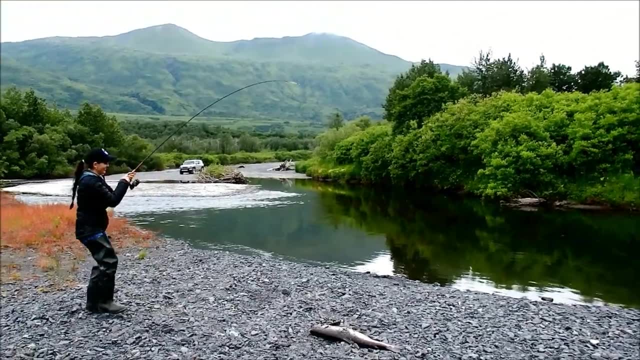 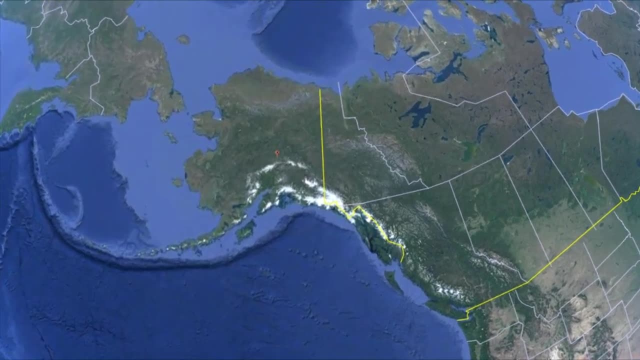 fishing alone. King salmon can be caught along rivers with spin fishing or fly fishing gear. No matter how you pursue the mighty king, though, you'll be in for quite an adventure, as well as some delicious, nutritious meals, if you're successful. Unfortunately, many king salmon populations are in decline these days due to a variety. 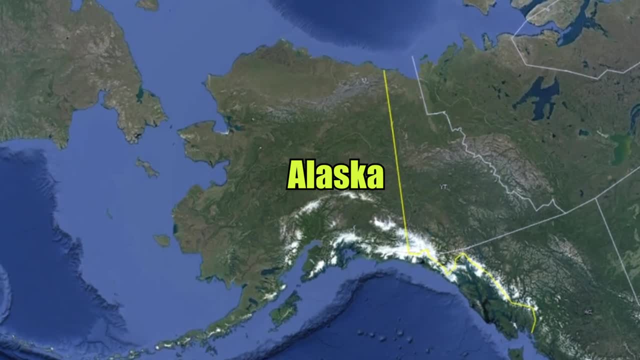 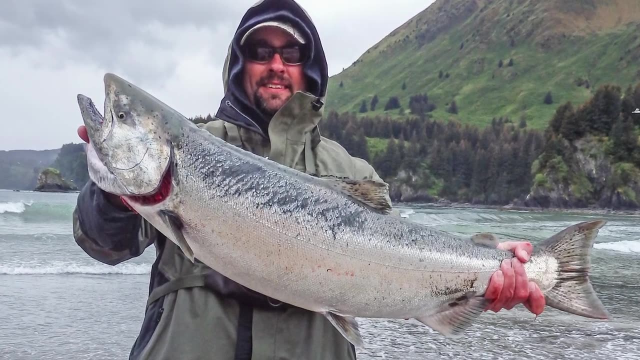 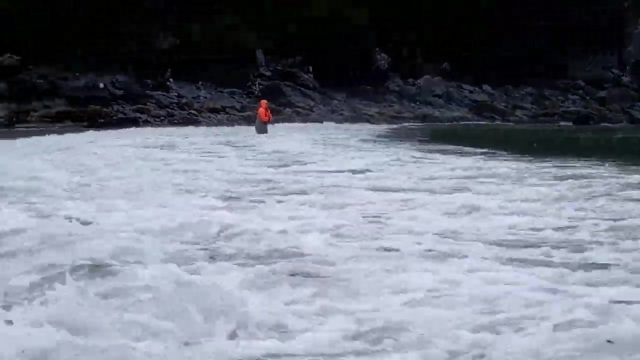 of factors. As a result, king salmon fishing is strictly regulated in places like Alaska. So those are some quick facts for you about the mighty Chinook. Now let's go fishing. Here's my good buddy, King Ron, landing a massive 35-pound king salmon while fishing.